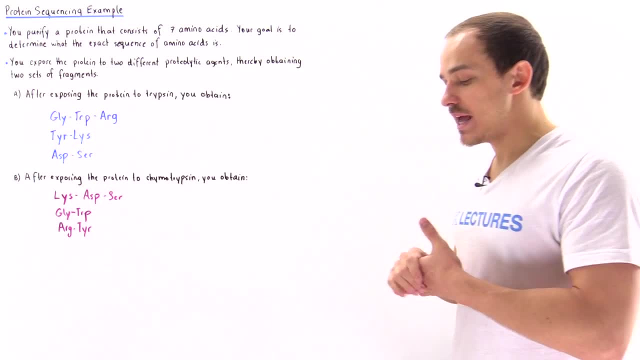 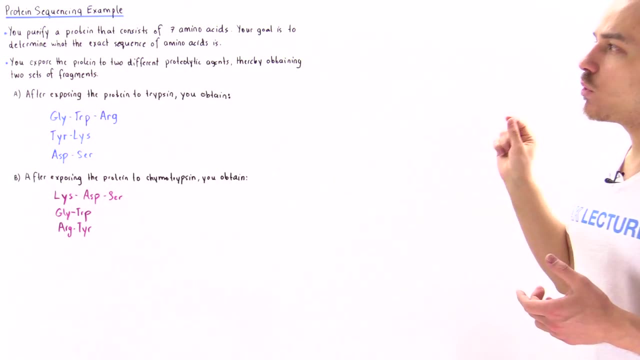 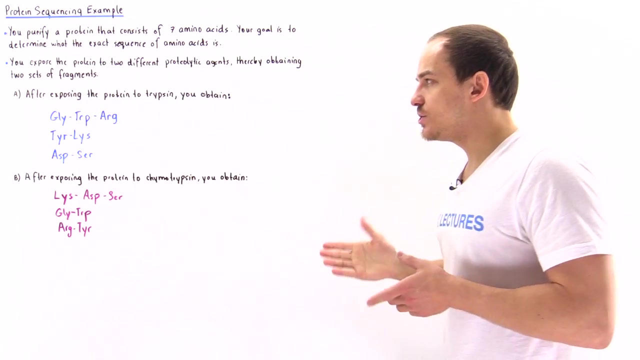 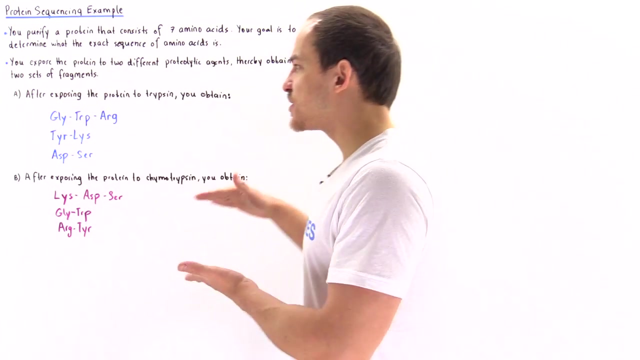 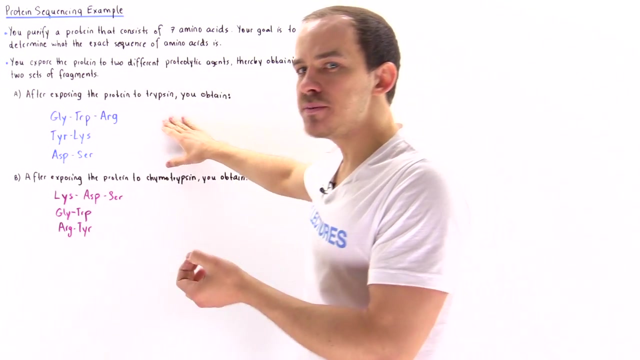 So suppose you purify a protein and that protein consists of seven amino acids. Now your goal is to basically find what the exact sequence of amino acids is in that given protein. And what you do is you expose the protein to two different proteolytic agents, thereby producing two sets of different fragments. So in experiment number one, you take your seven amino polypeptide, you expose it to trypsin, And what trypsin does, is it? 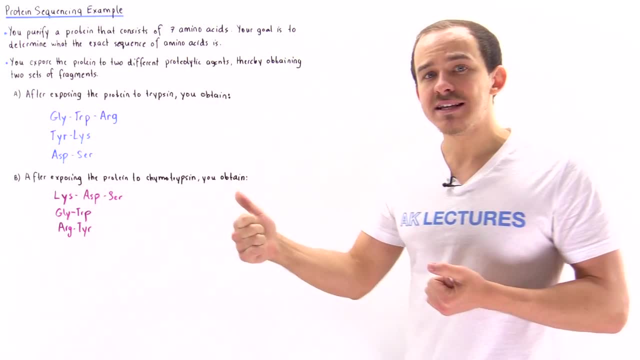 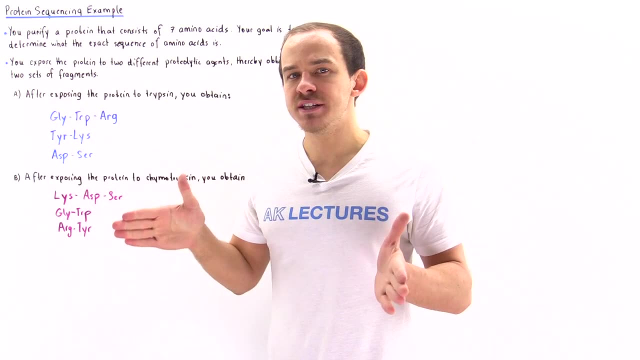 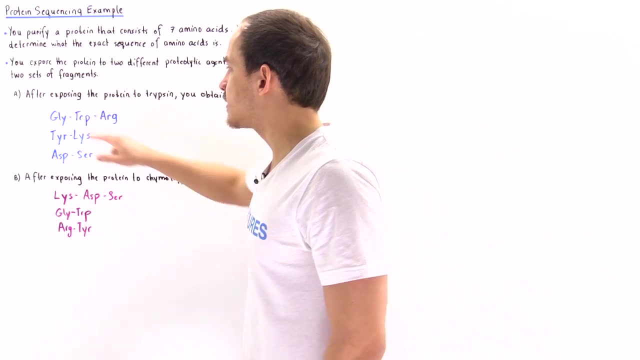 is a, a essentially cleaves at the carboxyl end of lysine and arginine, And what you obtain is these three fragments. Then you isolate these fragments and you conduct Edmund degradation on each one of these fragments And you find out that the first fragment is glycine, tryptophan, arginine. The second fragment is tyrosine, lysine, And the third fragment is aspartate and serine. Now you take that same polypeptide and you take the same- 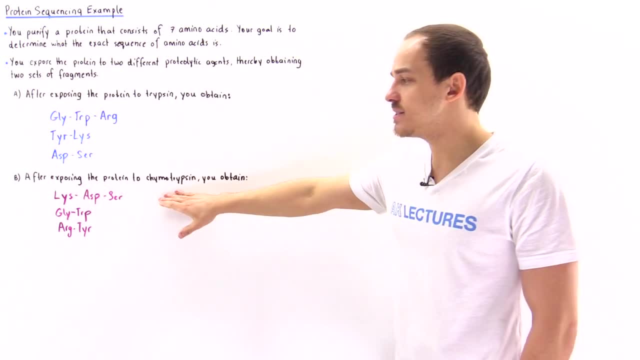 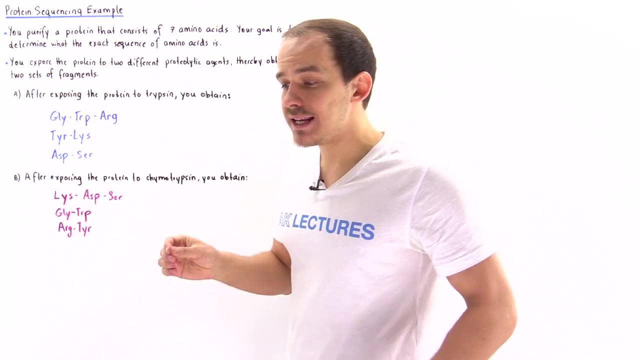 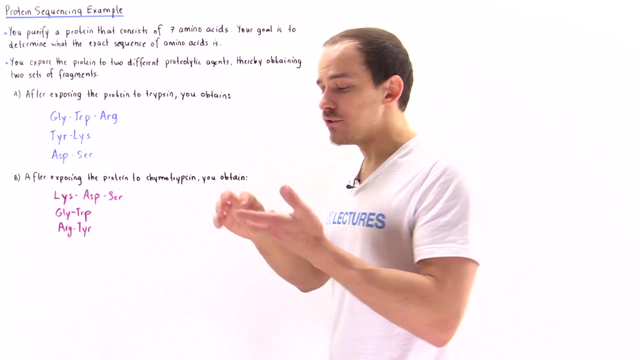 and now you expose it to a different proteolytic enzyme, in this case chymotrypsin. Now chymotrypsin cleaves our peptide at the carboxyl end of the bulky and aromatic amino acids, for example tyrosine, phenylalanine and tryptophan, as well as methionine and leucine. Now you get three. 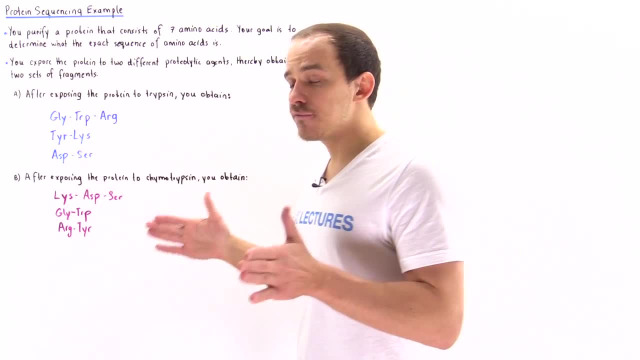 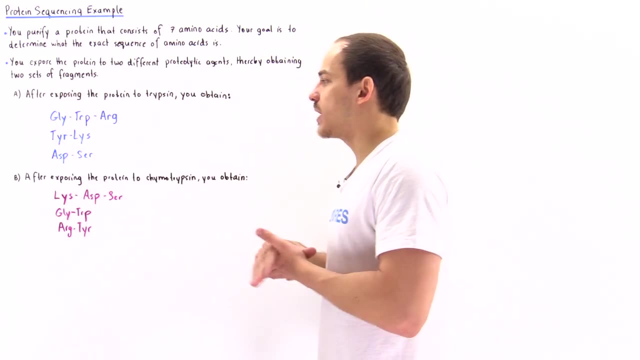 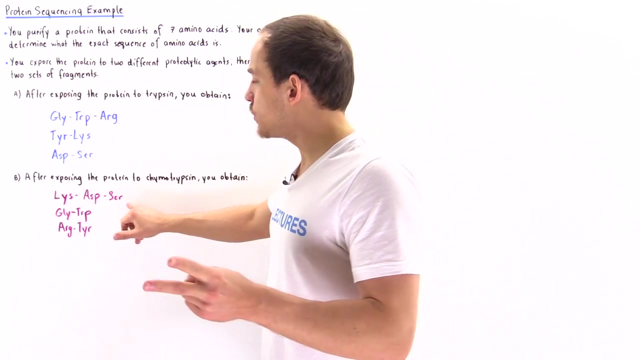 fragments as well and once again you isolate the three fragments and you sequence the amino acids in those three fragments by using the Edmund degradation process and you find that fragment number one is lysine, aspartate serine. fragment number two is glycine, tryptophan and 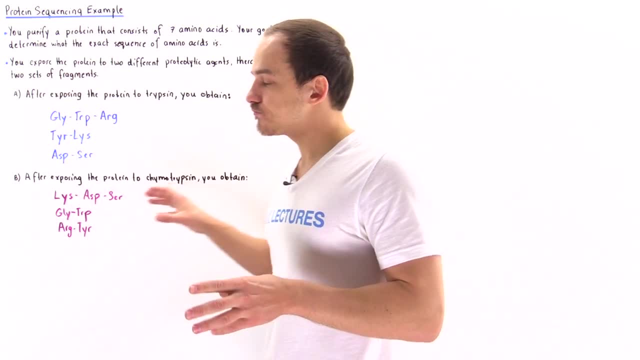 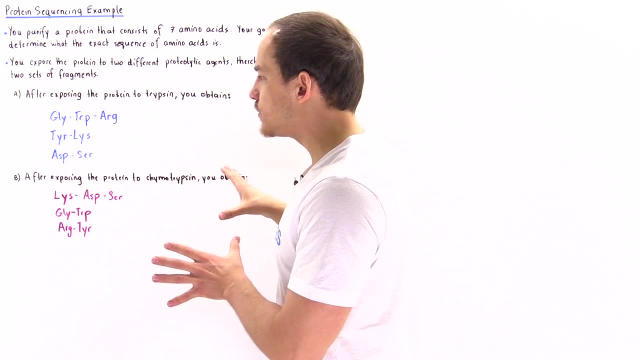 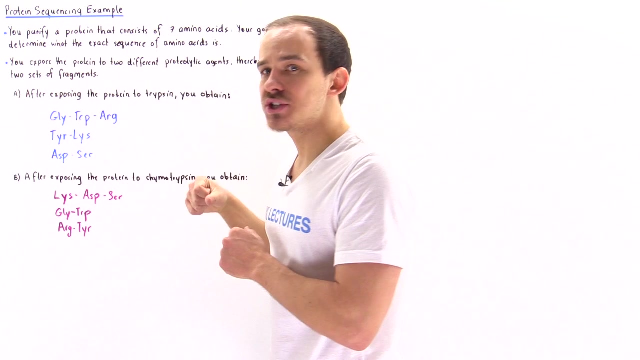 fragment number three is arginine and tyrosine. So now that you have these six different fragments- so you have two sets of fragments- you want to use the overlapping regions of the fragments to basically sequence the amino acids. Now the question is: are these fragments in the correct order with respect to one another? 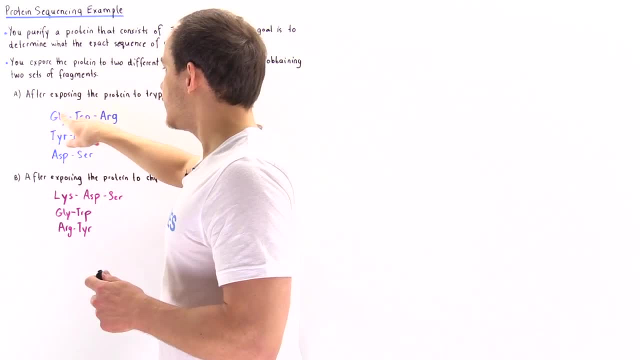 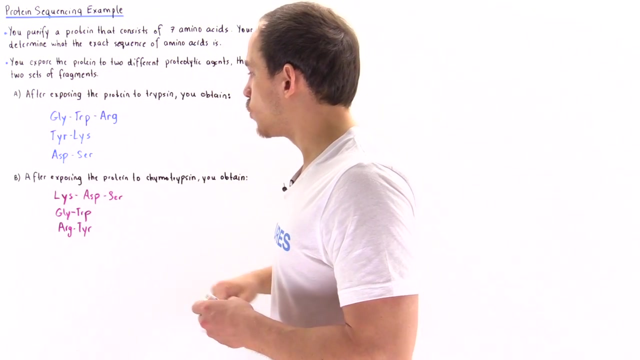 So let's begin on this fragment here. so we have glycine, tryptophan, arginine, we have tyrosine, lysine and aspartate and serine. So we only have a single glycine amino acid in the entire sequence. Now, if we look at the second experiment, where does our glycine 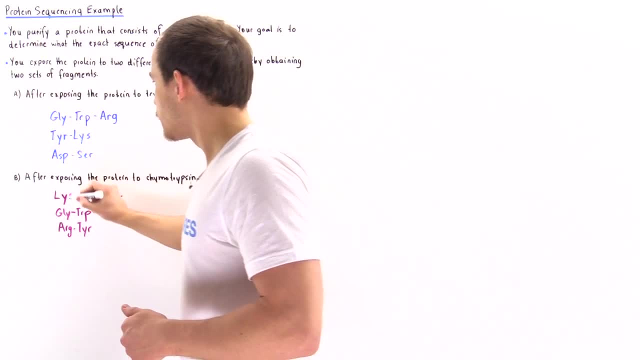 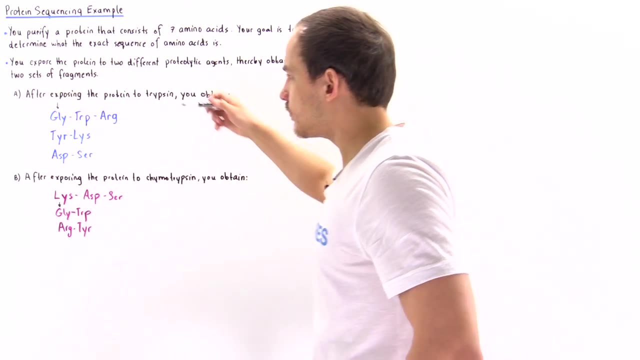 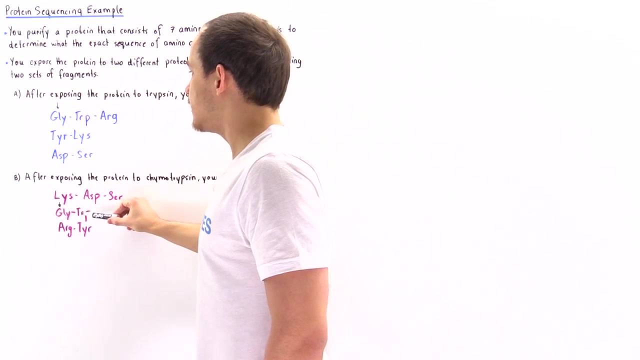 appear. So the glycine appears in the second fragment. here is the same glycine here, because we're dealing with the same exact peptide. Now, in this case we have glycine, tryptophan, arginine. In this case we only have glycine and tryptophan. So from this, 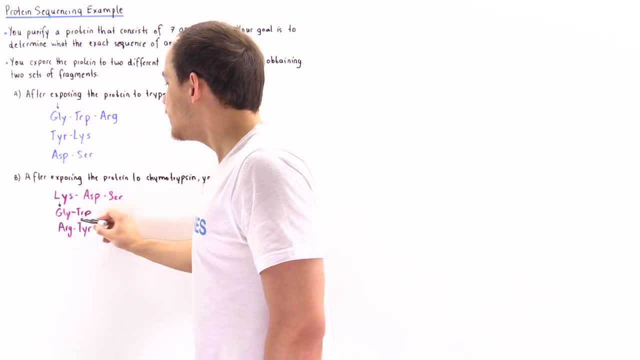 sequence. this arginine is missing. Now where does the arginine appear in these other two fragments? So this is our arginine, which is the same arginine as we have here. Now, in this case, nothing is attached onto this arginine, but in this case we have tyrosine attached to this arginine, So we know. 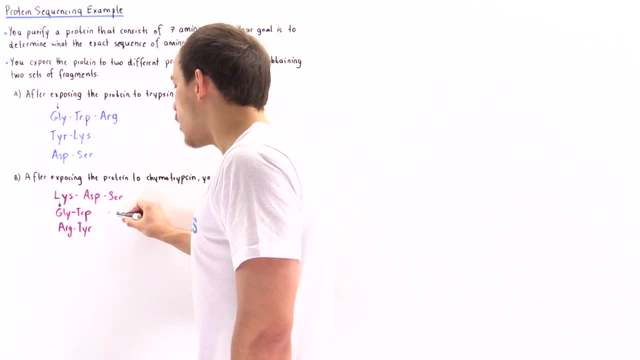 that the glycine, tryptophan, and then we have arginine. So this must be attached here, and because the tyrosine is attached to our arginine, we have glycine, tryptophan, arginine, tyrosine. Now the 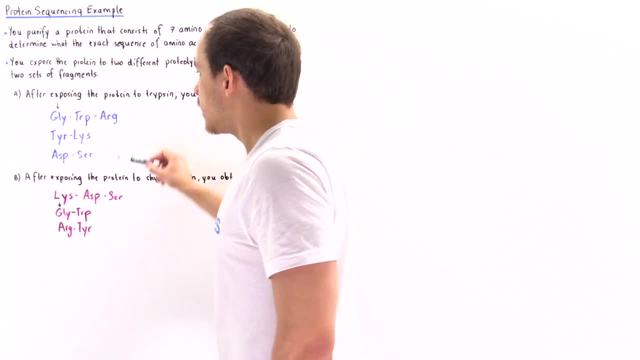 next question is: what do we put after tyrosine? Well, let's go back to this diagram here, to this experiment number one. So we have tyrosine appearing essentially right over here and tyrosine based on experiment one is attached to lysine, and the only time that lysine appears in this section is right over here. So we conclude. 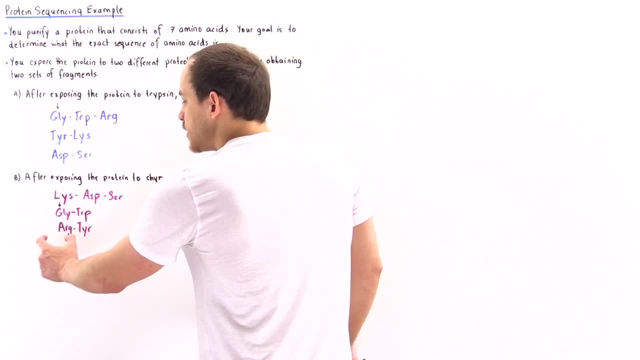 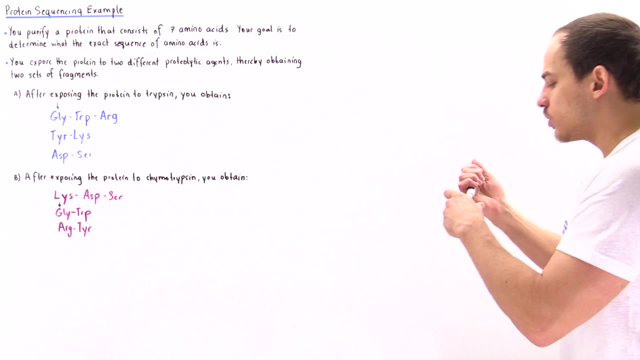 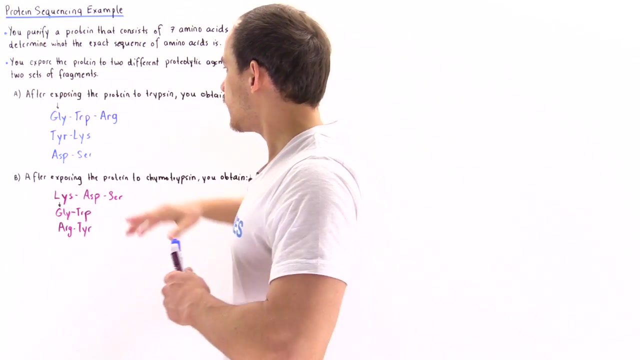 that we have glycine, tryptophan, then arginine, tyrosine and then lysine, aspartate serine. So once again, to see how all that works, let's take a look at the following. So let's actually write our result out. So let's begin with this fragment here. So we have, or 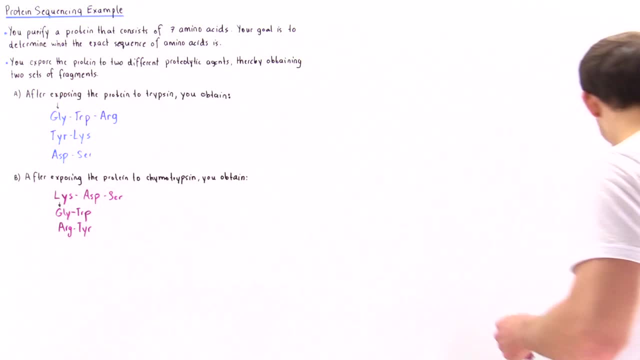 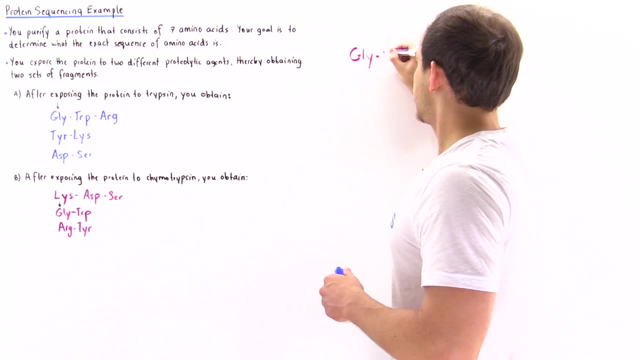 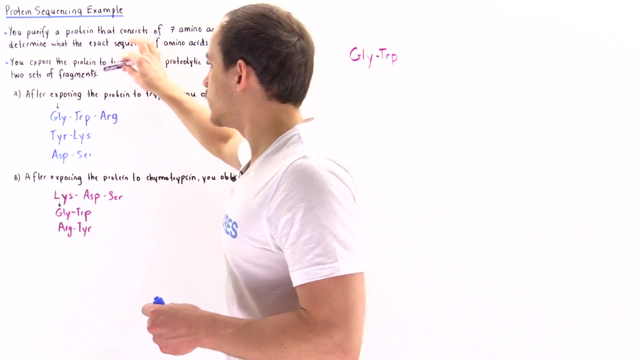 actually, let's begin with this one. So we have glycine and tryptophan. Let's use we have glycine and then we have tryptophan. Now to find out what comes next, we have to go to this experiment one. 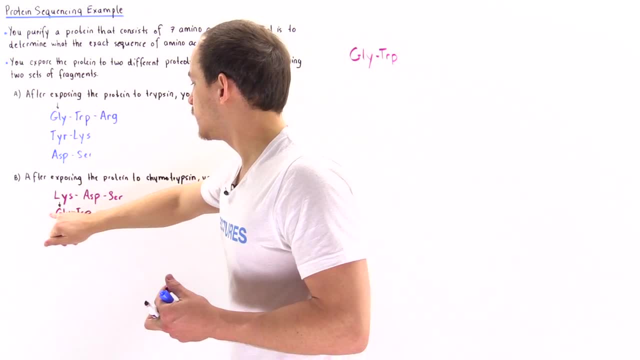 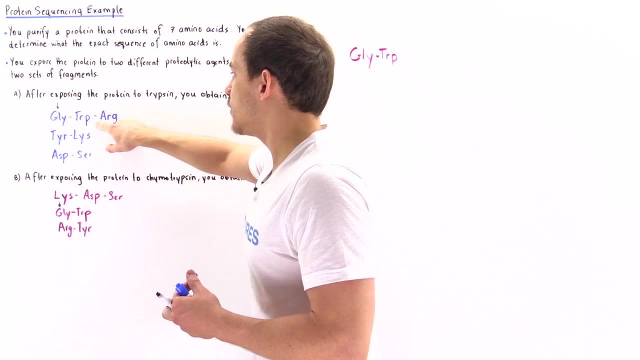 So we have glycine tryptophan, and the only time we have glycine tryptophan here is in this fragment: one glycine tryptophan, Now this third amino acid. that basically tells us which fragment must be connected. 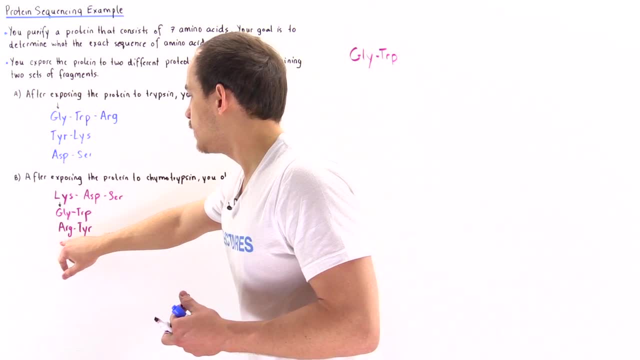 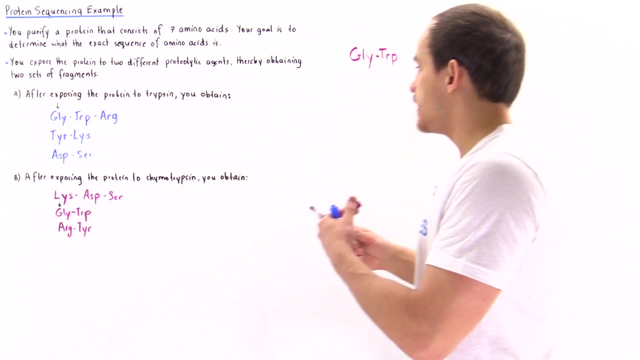 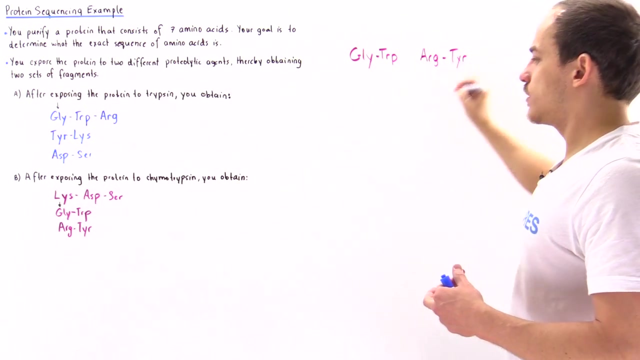 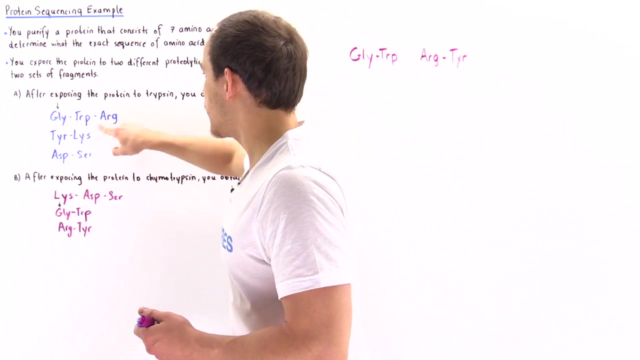 to this one. So we have arginine: appears in this fragment and nowhere else, And so that means the next fragment connected to this one is this fragment here. So let's place arginine and tyrosine- the third amino acid, third fragment- here, And then we have arginine-tyrosine. so we have arginine and the only place where 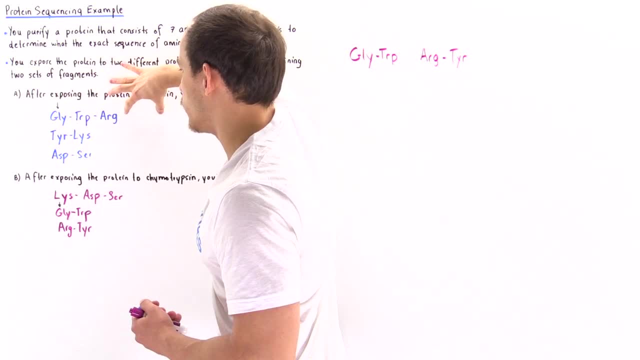 tyrosine appears is here, So we have tyrosine, should go here. we have tyrosine-lysine and the only time we have tyrosine and lysine, or the only time we have lysine, in this case. 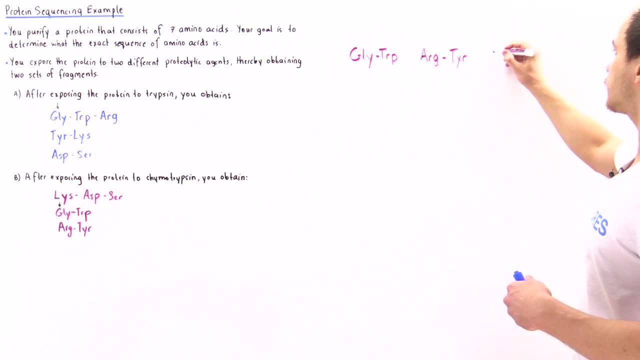 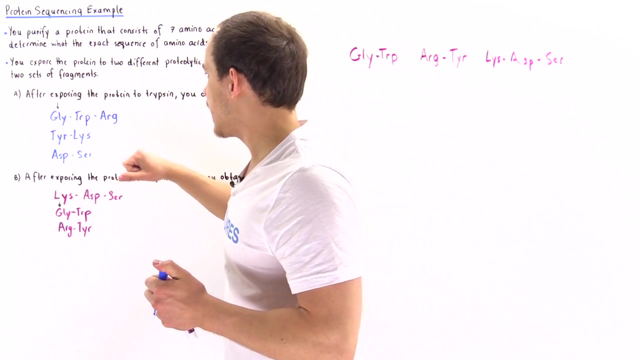 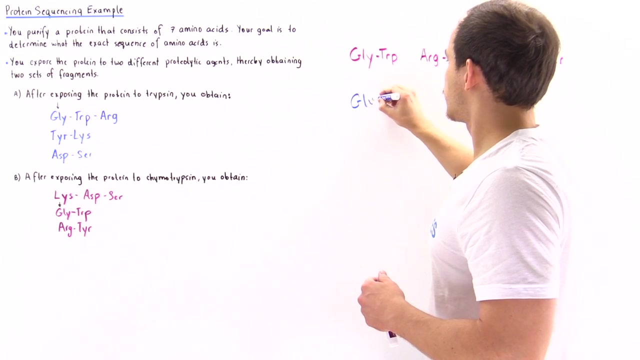 is in fragment number one. So we have lysine, then we have aspartate and we have serine. Now let's place these underneath this row. so we essentially have our glycine, tryptophan, arginine, which basically appears here. So we have glycine, we have tryptophan and then 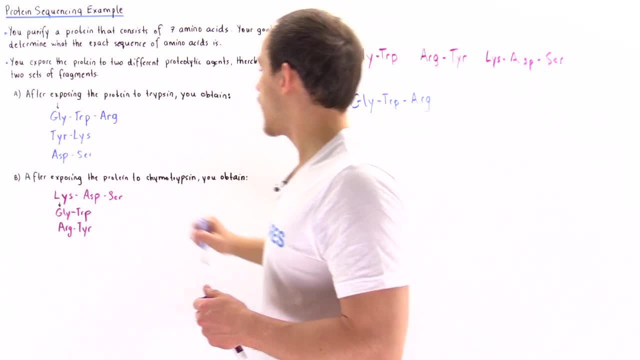 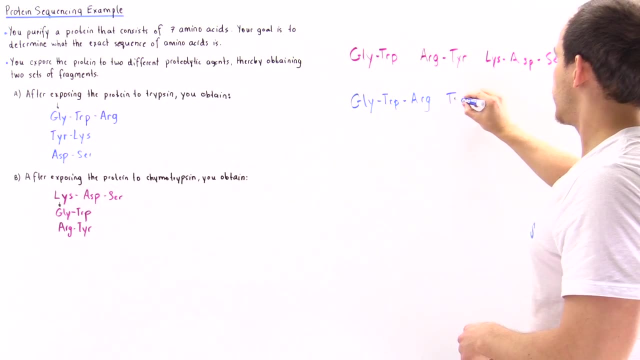 we have arginine. we have these two fragments, So we have tyrosine lysine and we have tyrosine lysine. So let's put that here: We have tyrosine lysine and the final fragment is aspartate serine, which are these two. 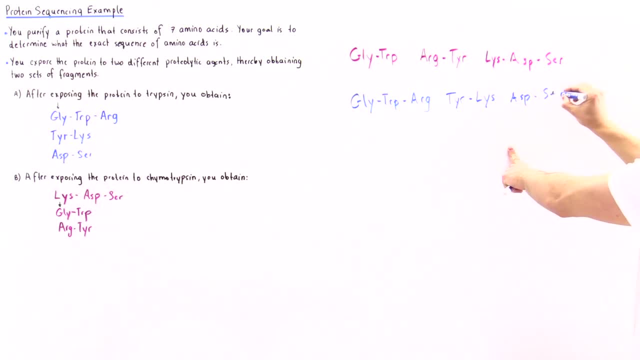 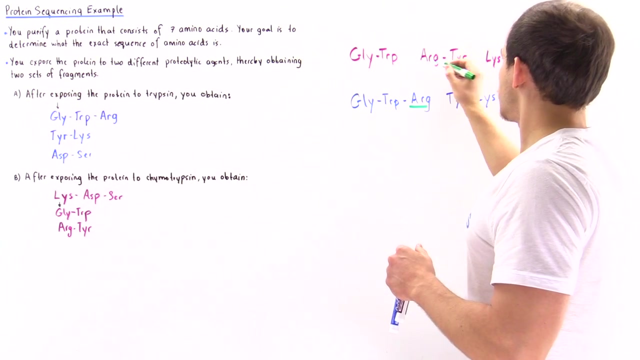 amino acids here, So aspartate and serine. Okay, So we can piece together these overlapping sections. So let's use, let's say, the color green to basically describe the overlapping section. So we have, we have. what do we have here? We have arginine, which is right over here, right, And we 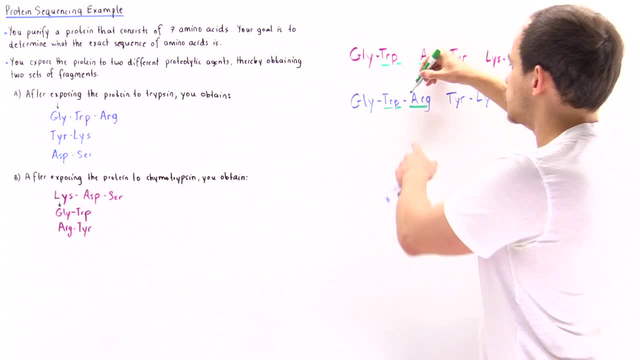 have tryptophan, which is right over here, And so there should be a bond right over here. And likewise, we have arginine and tyrosine right And arginine- tyrosine, So there should be a bond over here. 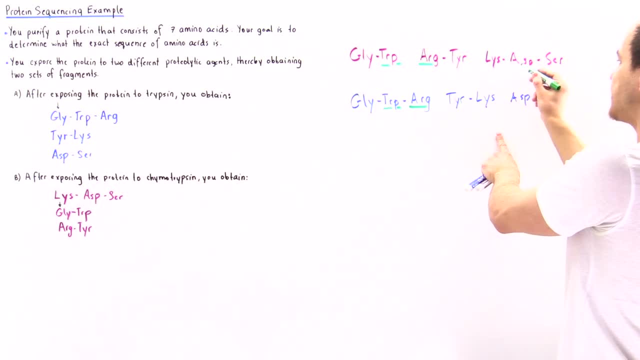 Here. If we look on this side, we have lysine aspartate and this is lysine aspartate. So there should be a bond here. And tyrosine lysine tells us that tyrosine lysine- there should be a bond.